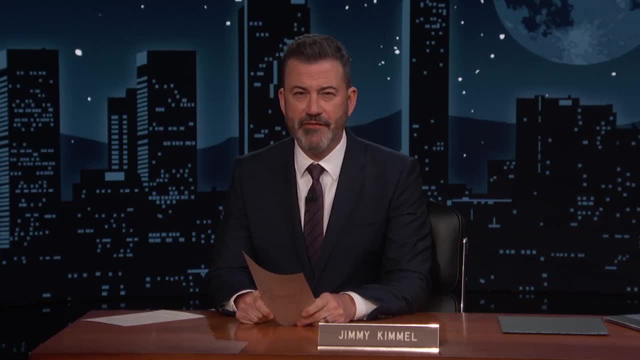 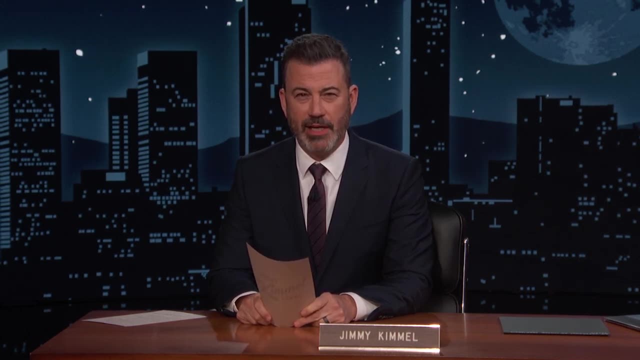 Our first guest tonight is one of very few Emmy Award-winning actors who can carve a canoe out of a tree. He plays a dystopian president in a dystopian America in the number one dystopian movie in the country- Civil War- is in theaters now. Please welcome Nick Offerman. 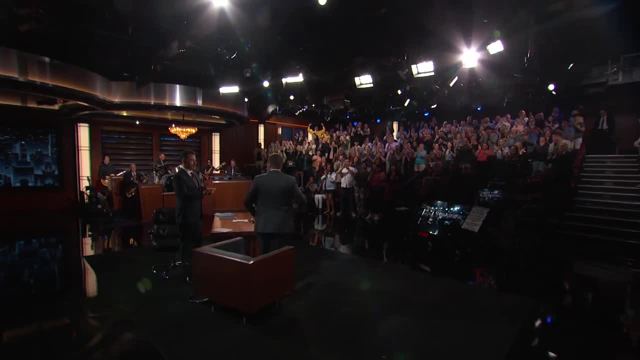 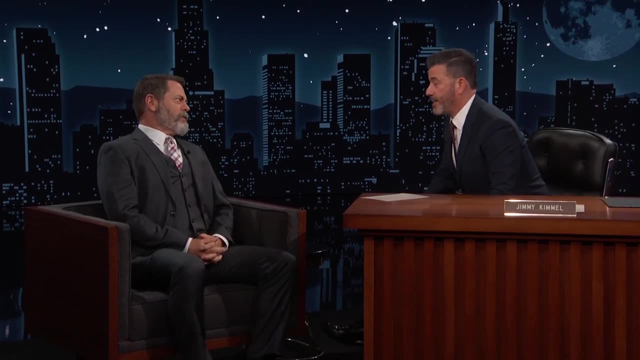 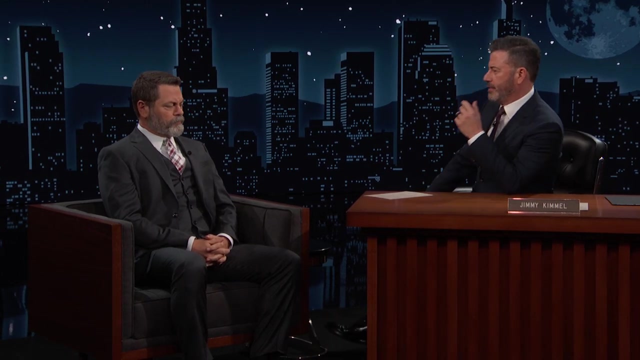 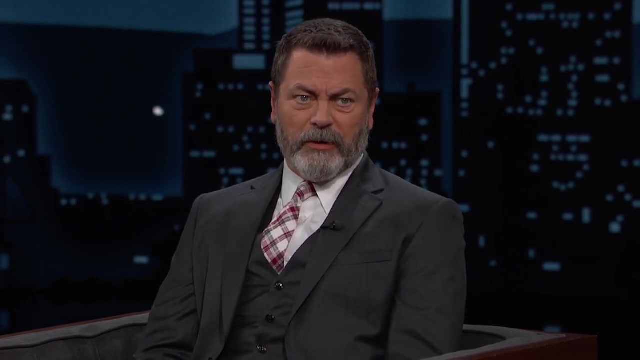 Well, may I begin by saying that was one of the finest portrayals of Arizona territorial lawyer somebody, T Howell, I've ever seen. Yes, Thank you very much. Blessing with us. I'm classically trained at the University of Illinois, so I hope I did them proud. 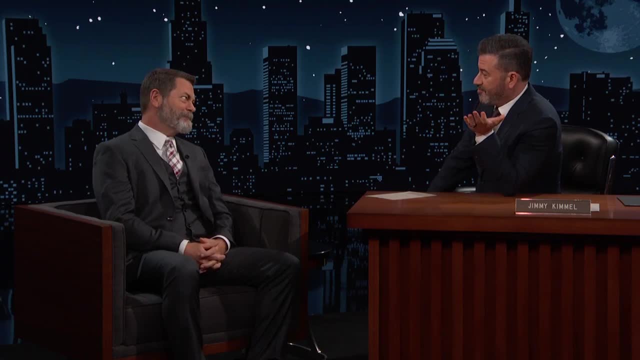 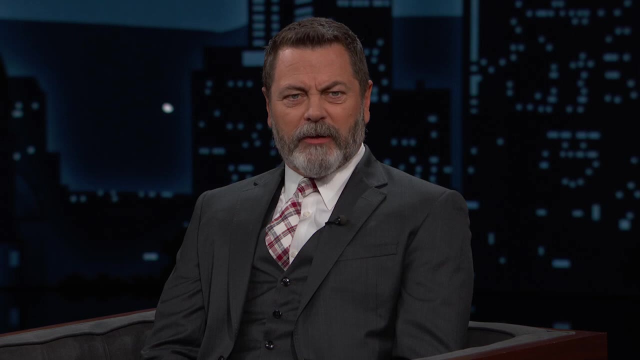 You did. You certainly did, And I know that you come from a family. You come from a family of politicians, which is something I learned today. I do. I mean, they would argue it's a bit of a stretch, but my grandfather was the mayor of our small Illinois town, Manuka, back when I was a kid. 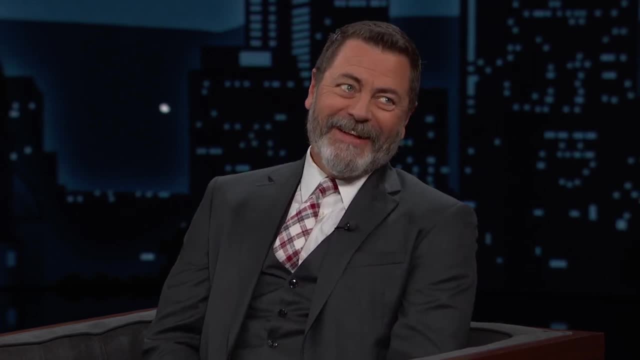 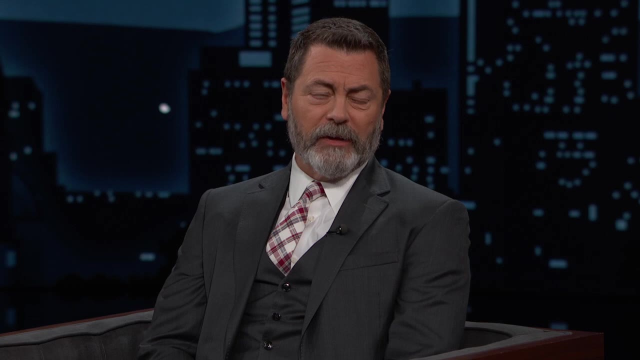 And then my dad is now the mayor And so people always say to me, and so I say: my sister, who's a very powerful librarian, I think, Is she. She will probably be next in line, hopefully. Is your sister really a librarian? 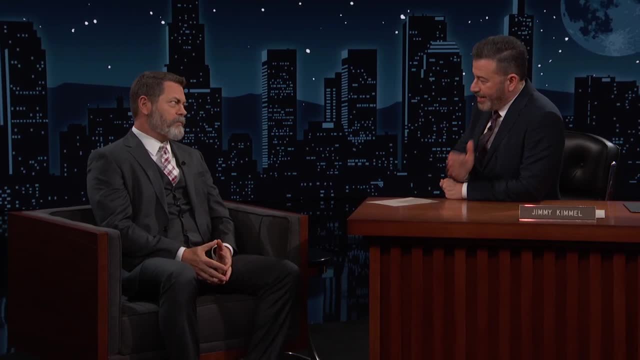 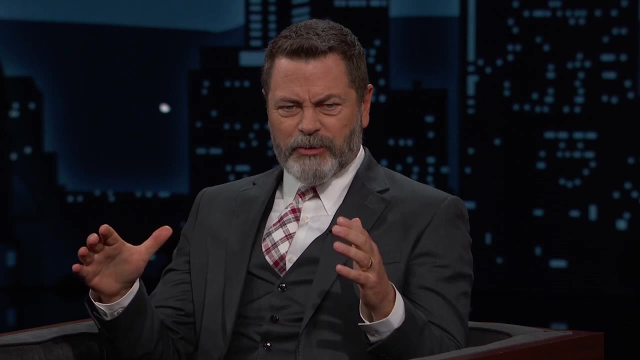 A very powerful. And does she work in the library? She's there with the Dewey Decimal System and the whole deal. That's right. yeah, Well, she controls. She worked her way up, so now she's sort of like a mafia don. 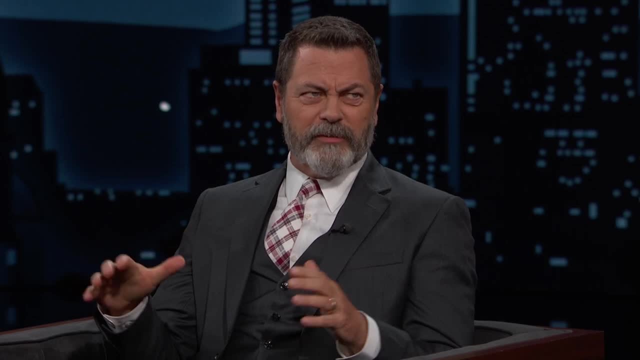 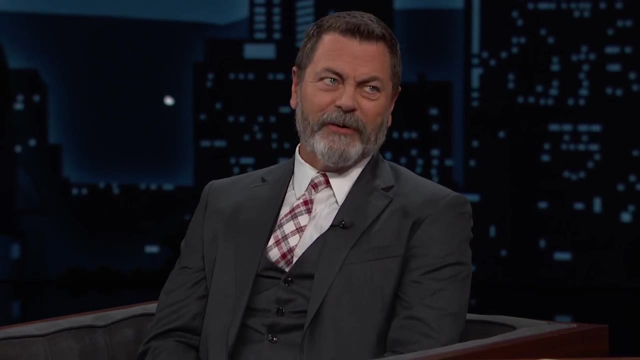 She oversees a region of Illinois libraries, the Three Rivers Public Library System. I hope I can say that I hope so too. She's very intimidating. When you write a book, does she see to it that it gets preferential placement, or does she see to it that the book is not available? 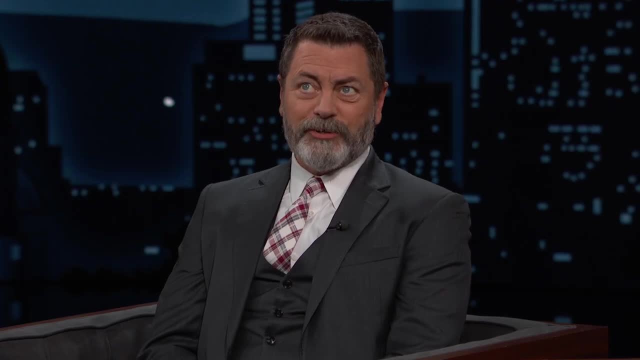 Well, I think that's a very astute question. Most of my books have pride of placement, but the one that talks about my siblings I haven't seen yet on the show. Oh, All right. Well, maybe you put in a word with your sister. 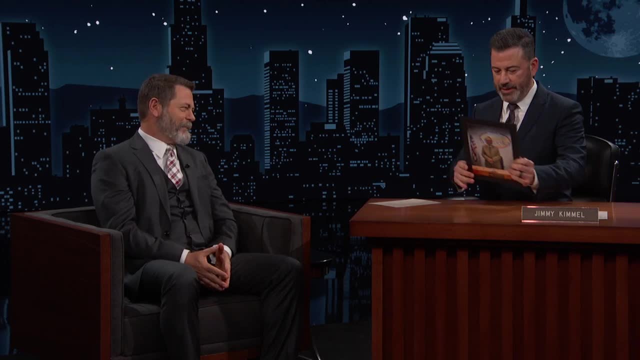 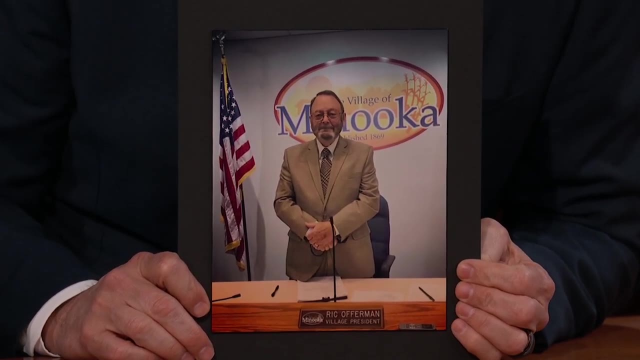 So your dad? I have a photo of your dad. I think this was from when he was village president of the town- is Manuka Manuka? The way he's standing here, it looks like mooka. I mean, I don't know. 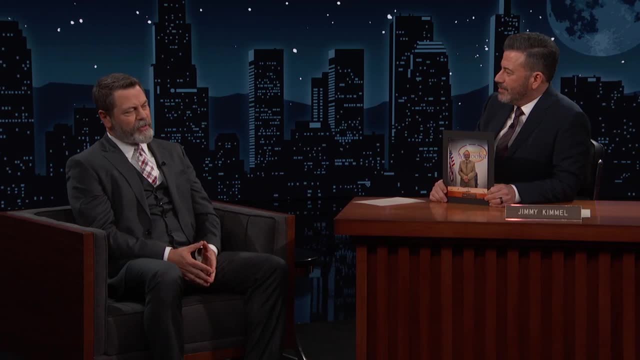 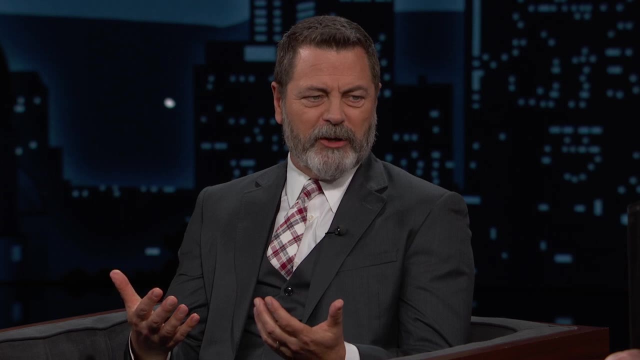 What makes it a village, by the way? What is the? you know? That's a great question. A village versus a town? I mean it must be a population thing. Yeah, Growing up there were just a couple thousand people, but now the commuters of Chicago have found us, so now we've got a stoplight. 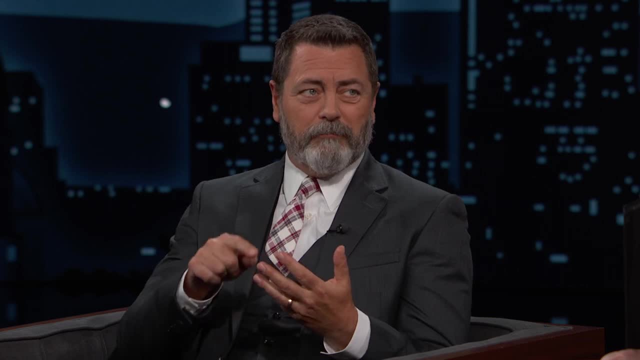 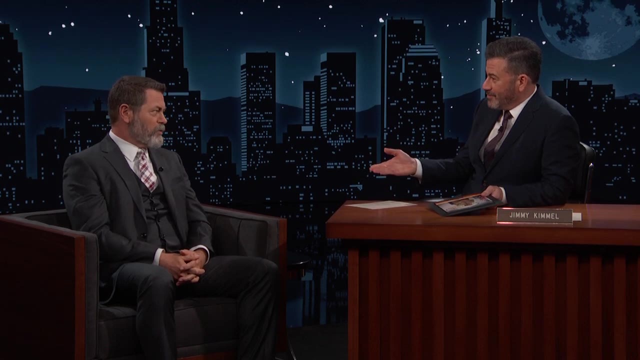 You can get bread. You can get meat, bread and condiments all in town. You no longer have to go to Jule. When you were growing up you had to actually travel to get those things. We had to make our own mustard. 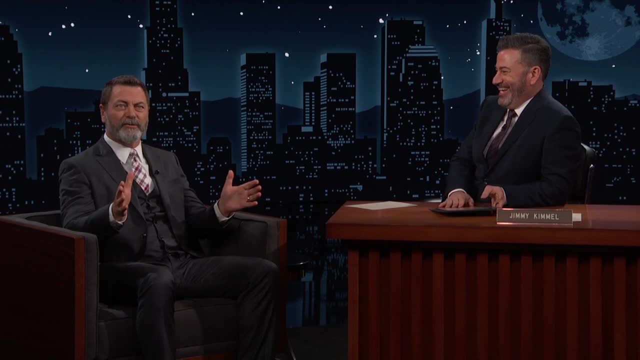 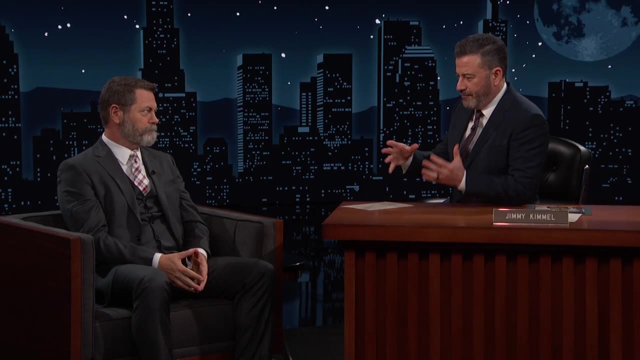 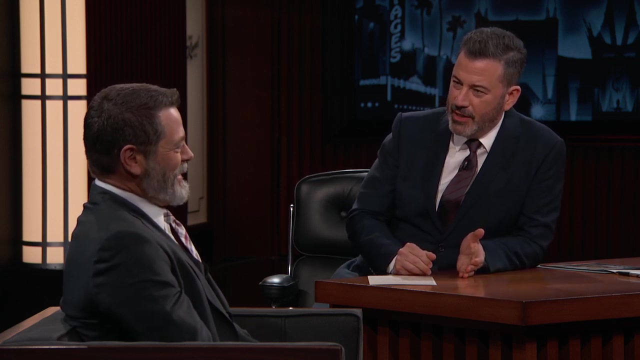 That's not a euphemism- You so, when your dad, your grandfather, et cetera are involved in the, you know, town, council or whatever, do you have to behave yourself? Is like there extra pressure on you as a young man? 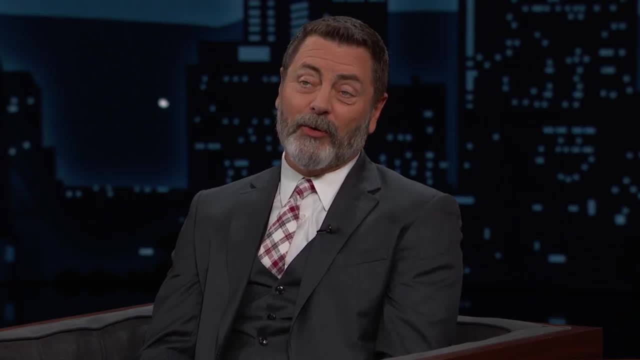 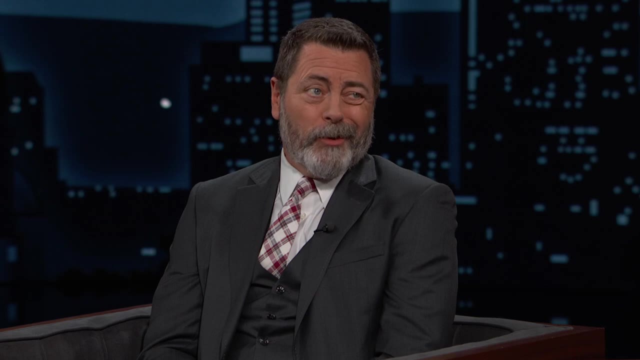 You would think I mean, this is America, And so what I've learned from the example of others is that if your family's in power, you maybe get away with it. You might get away with it a little more. Oh, the opposite. 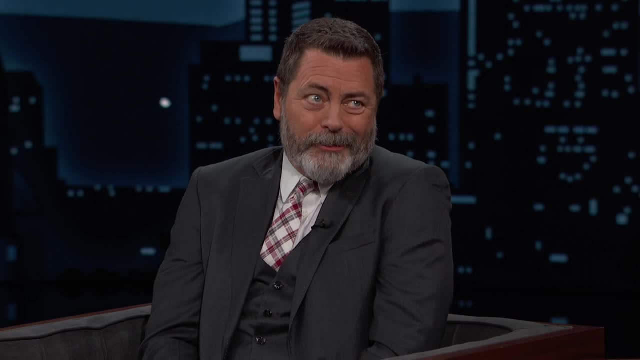 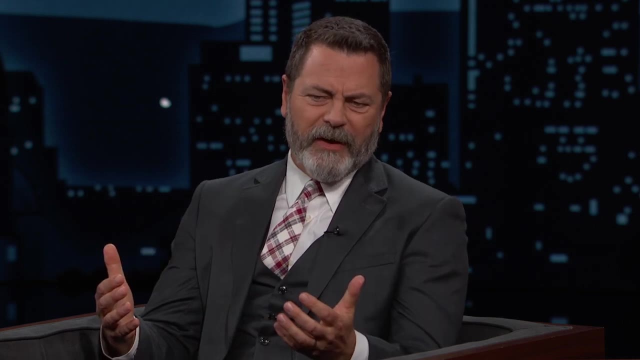 Yeah, Saudi Arabia might send you a couple billion dollars if you play your cards right. I was the black sheep. I have this wonderful family. There are 40 of us around. Manuka and Megan and I are the only two that don't live there. 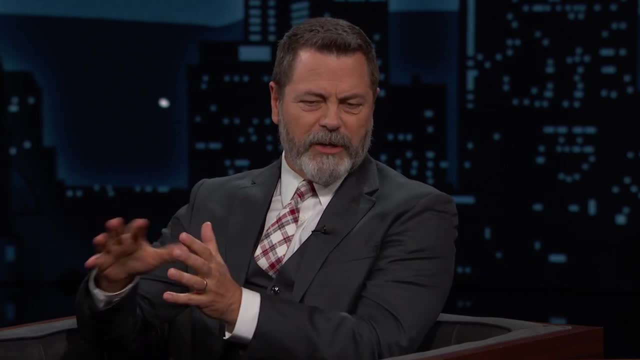 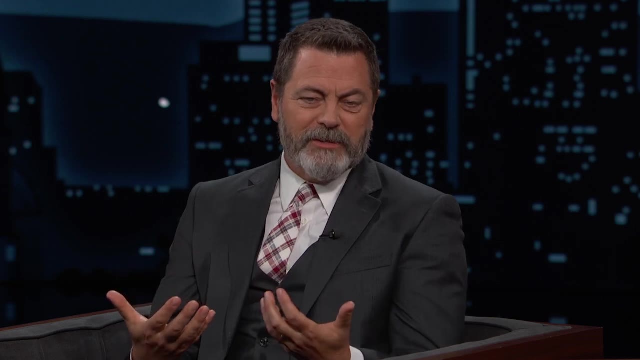 Is that true? Yeah, It's this incredible. half of them are farmers on mom's side. and then we have the mayor, We have school teachers, librarians, paramedics. They're exemplary citizens. And then there's There's one douchebag. 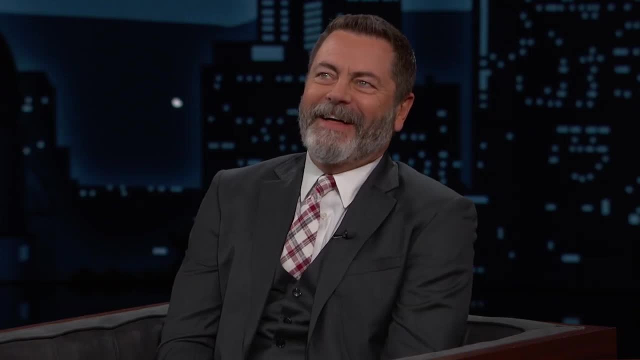 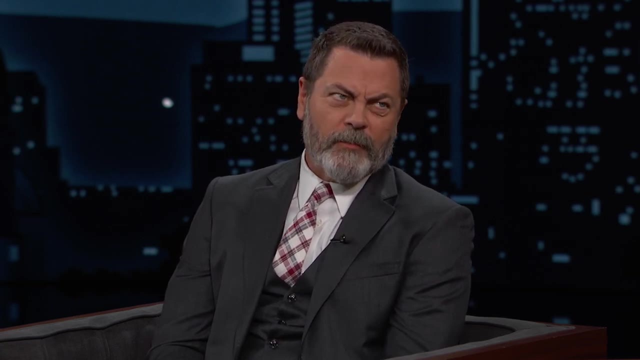 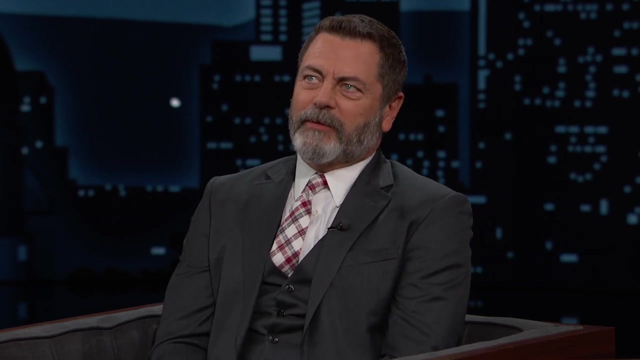 And what about me? And so I experimented with misdemeanors when I was young, But please detail us. What did you do? And remember you're among friends. I mean, these were great lessons learned When I was in college. my friend and I had a game. 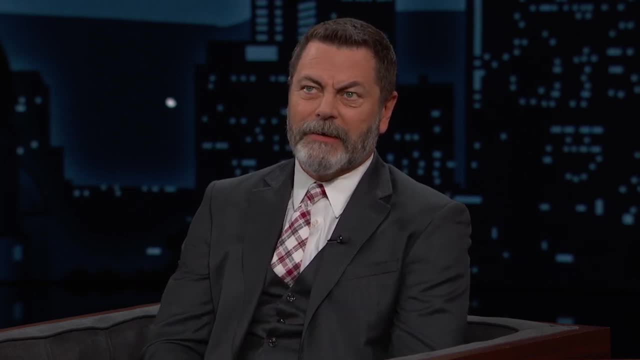 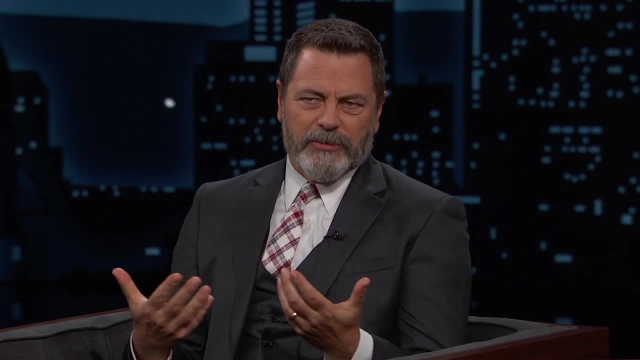 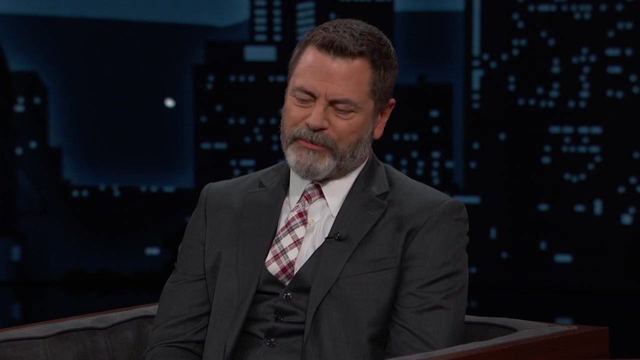 And talk about the privilege of the bourgeoisie. We had a game where we'd go. We'd go into a store and steal the dumbest thing we could to make each other laugh. So it was shoplifting as a diversion And I got caught in a Kmart, which is the place where they're watching for shoplifters the closest. 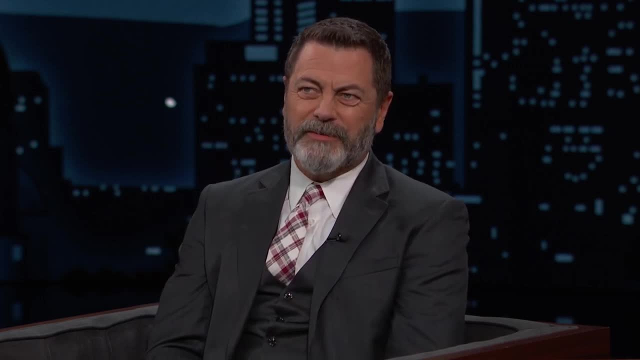 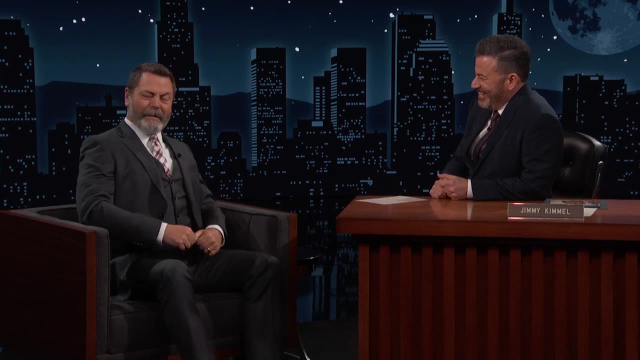 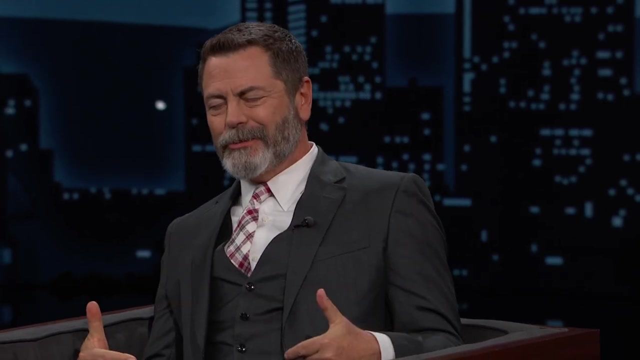 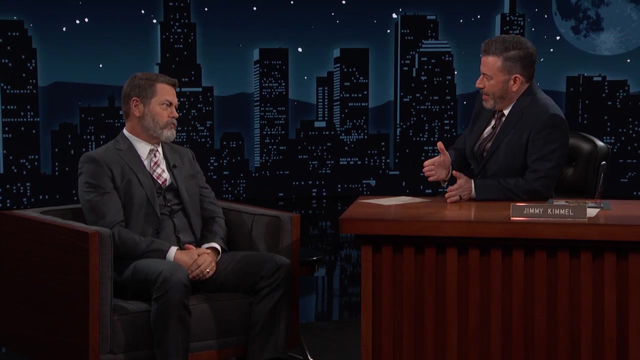 Sure Shoving eight Ronnie Millsap cassettes down the front of my jeans And walking out. Just couldn't wait to see the look on Joe Faust's face when I was like, check this out, Ronnie Millsap, Were they all the same album? 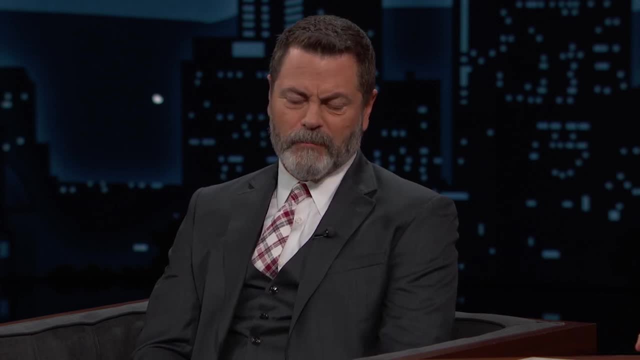 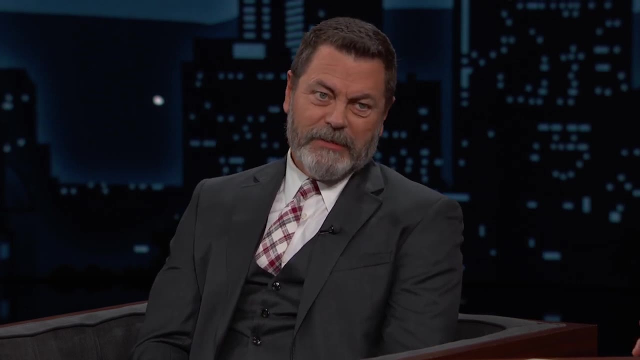 Eight different records. Oh, eight different records. Oh, you got his whole catalog down there. It was the perfect crime, Until it wasn't. It was scary. I went to jail And I was terrified. You went to jail for stealing Ronnie. 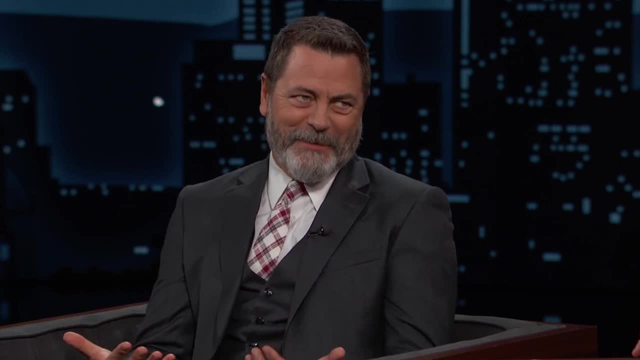 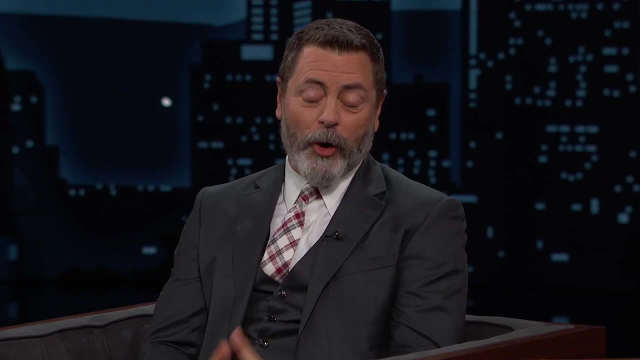 Ronnie Millsap. Yeah, And I was like, come on, you guys. Clearly this is a bit, But they wanted to teach me a lesson And they did. It was the opening night. It was the opening night of the first time I got cast in a play at the University of Illinois. 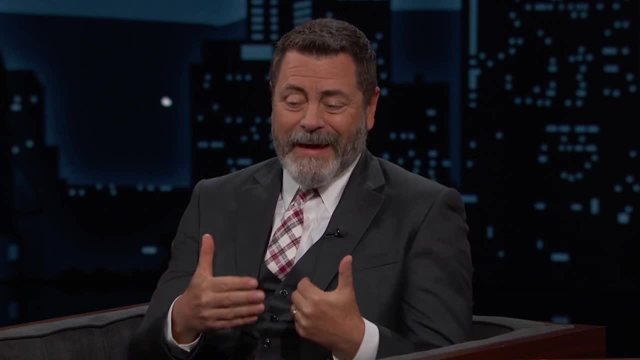 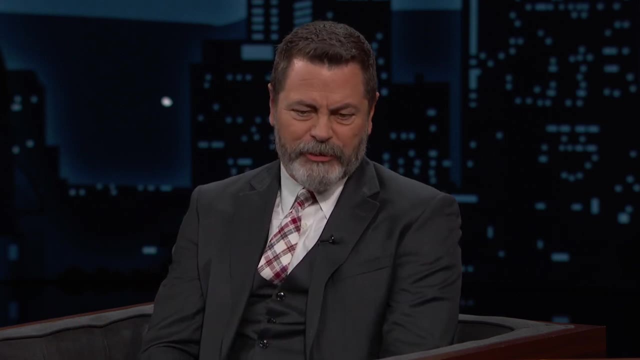 And I was in this production of Picnic, And so if I hadn't made it to the play I probably would have been kicked out of school. But a friend of mine- his name was Rob Taich- came and bailed me out. 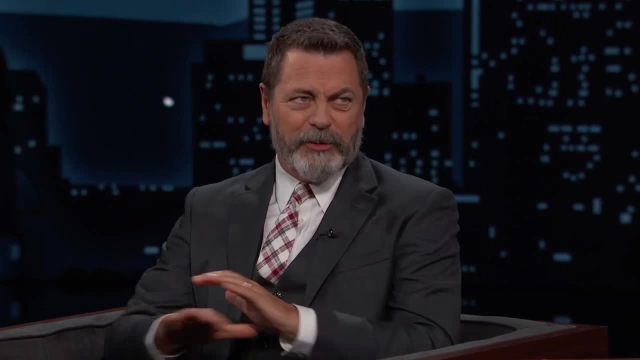 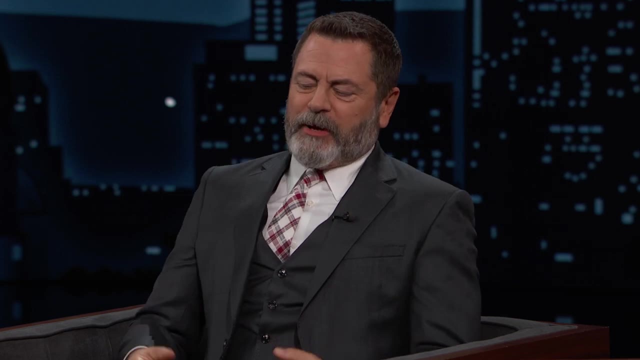 And my other friend was the assistant director. Nobody knew, Nobody told anybody. Twelve minutes before curtain I got to the theater and, like, put on my stuff and went out and gave the most tearful performance of it. Was that the? 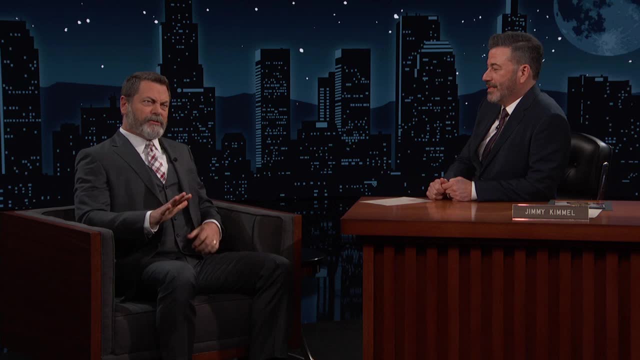 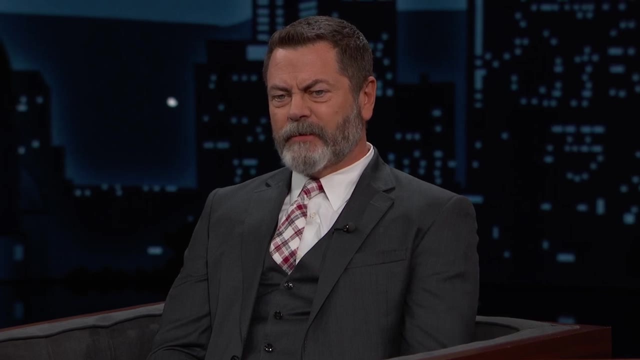 That's a pretty good cry. My mom and dad don't know about this. Was that the end of it Or did Joe keep going? I don't know. There was one other time, I don't know, In the Urbana jail. 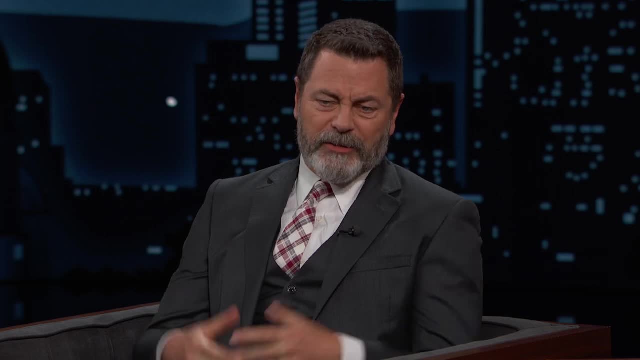 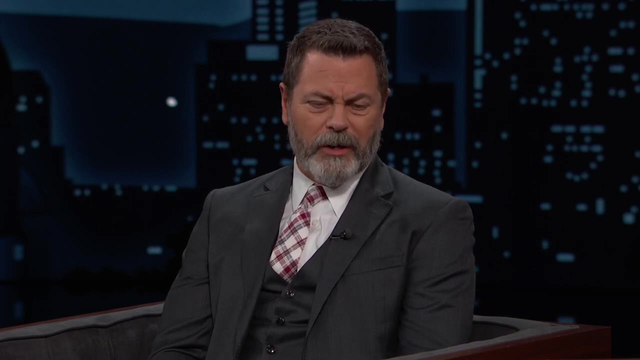 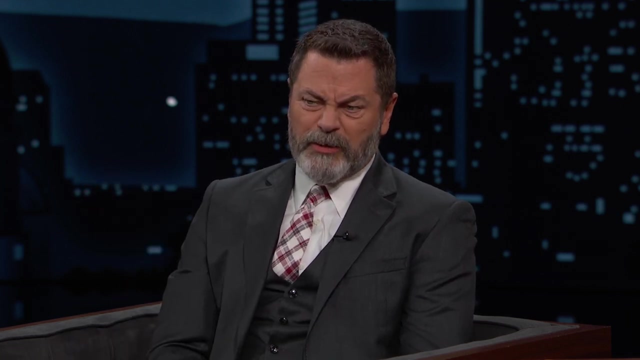 Some friends and I- we can say this now- in California- we were smoking marijuana out behind a community theater late one night And some flashlights came along the creek where we were hanging out And we realized it was police, And so we began to tiptoe away. 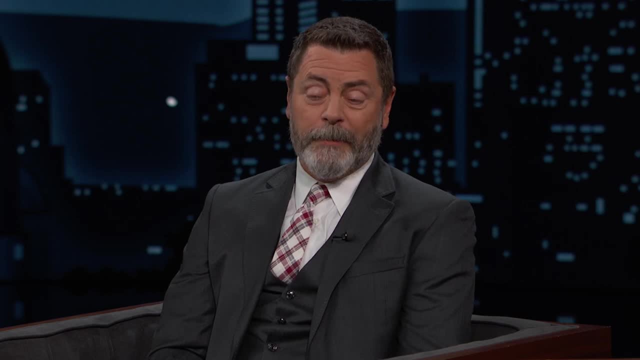 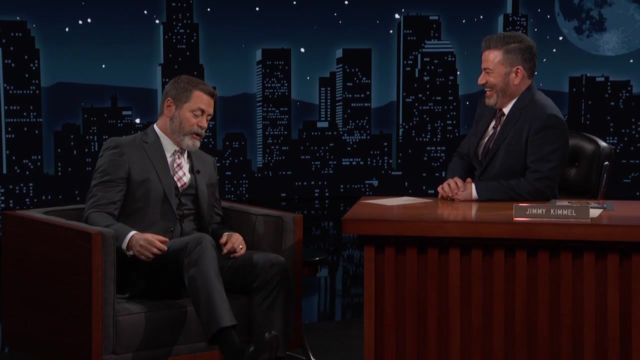 And they gave chase And we wisely ran And they tackled us And an incredibly tough, diminutive woman who I think may have been Holly Hunter. I couldn't tell because she had her boot on my head and she had her gun on me. 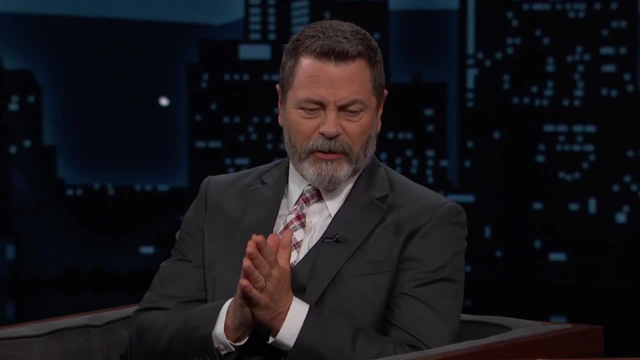 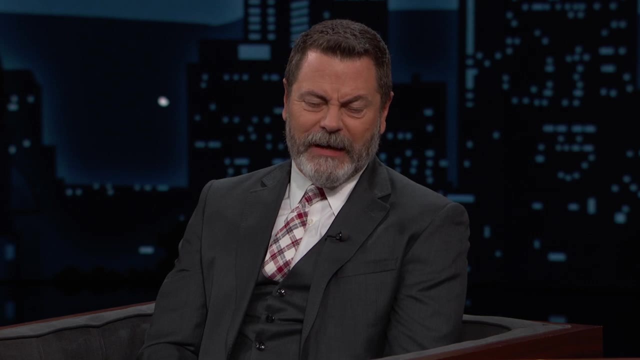 Oh boy. So they tackled us in a parking lot And it suddenly got incredibly real And we said: I don't think we did whatever you think we did. This has suddenly gotten out of hand And it turned out that a restaurant had been robbed of a bunch of cash up the creek. 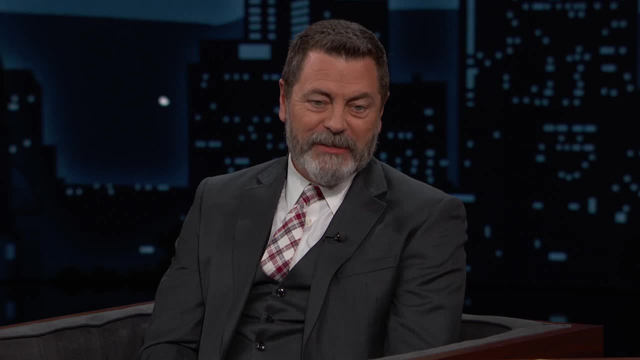 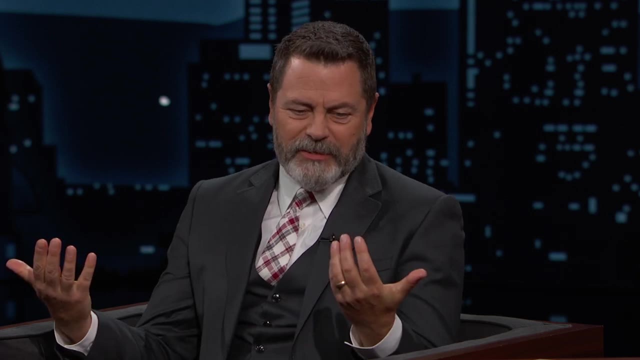 And so they, naturally they saw these kids running And we spent the whole night in jail. Oh, And the thing is, we were just these innocent dumb theater kids And we were saying, no, we were just out there smoking and talking officer. 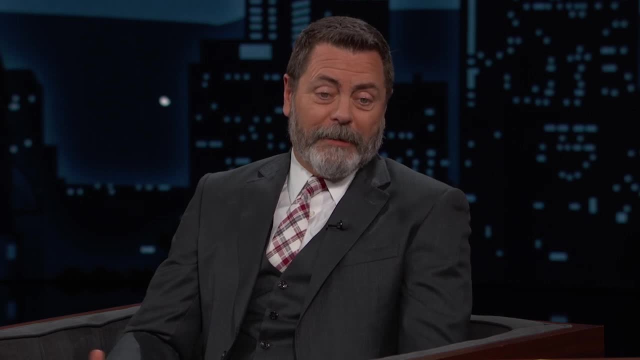 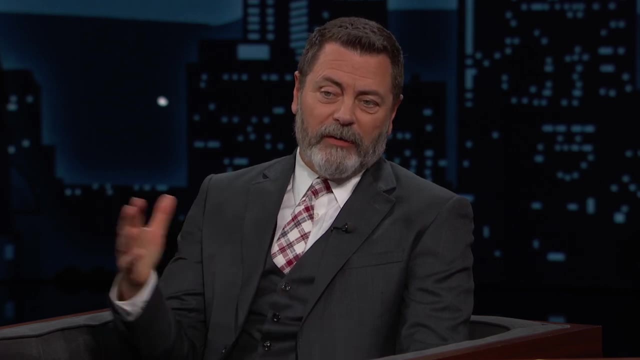 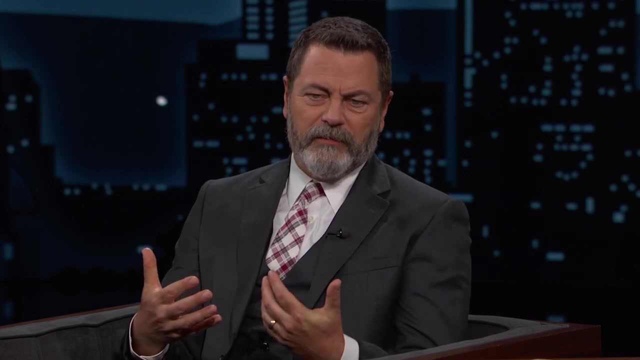 And I'm too f***ed to drunk. It usually gets you off. You know they love that joke, Uh-huh, yeah, sure, And thankfully we did. We put up enough of a collective front that they decided we weren't the thieves. 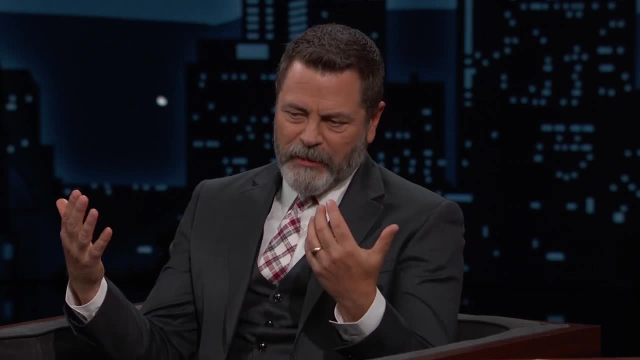 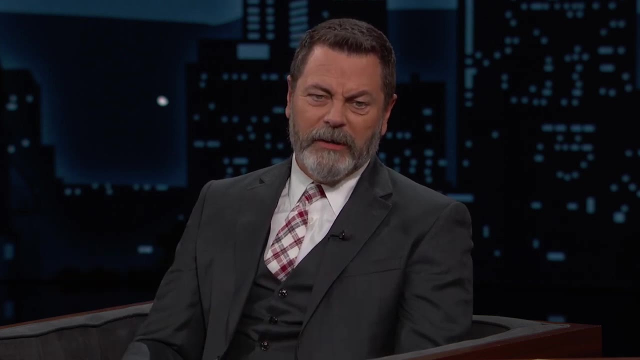 They let us go in the morning, So they kept us all night And as the sun was coming up we walked out And on the front lawn of this sheriff's station, my friend Greg, who had the one-hitter, the pot-smoking paraphernalia- 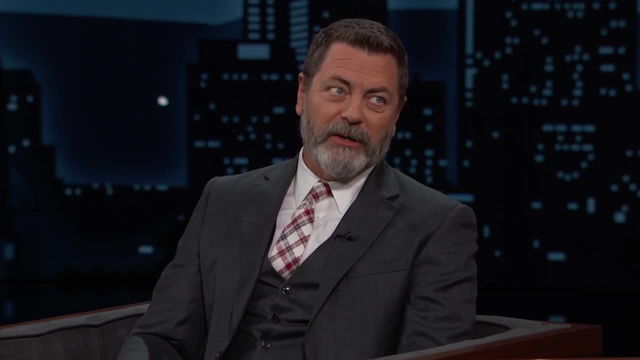 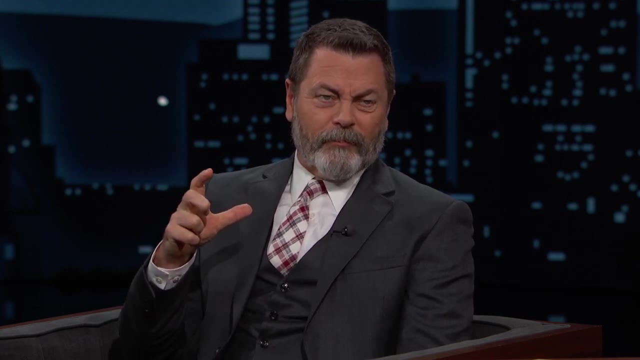 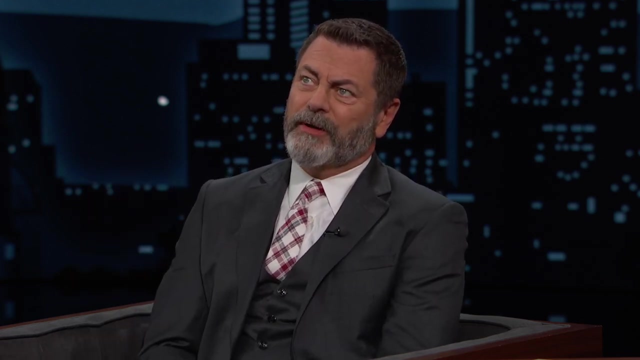 we said it's a bummer that you had to throw that in the creek when they were chasing us. And he reached into his crotch and pulled it out and was like you think I'm going to throw this. And so we smoked marijuana first thing in the morning in Urbana in front of the sheriff's station. 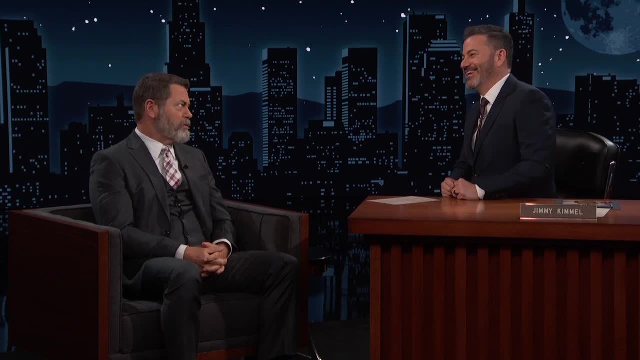 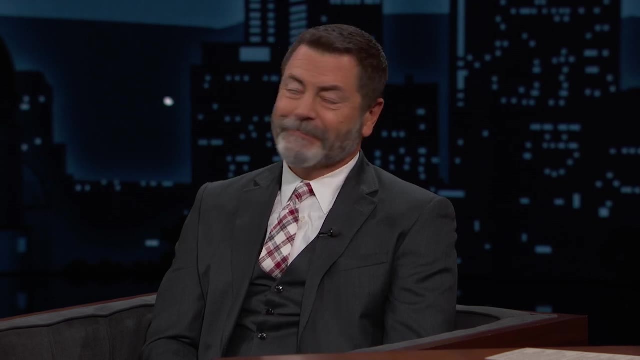 And now here I am. Wow, that's. I mean that's. If you want to make it in showbiz, you could do a lot worse. You reach down into the pants, you pull out a one-hitter. maybe there's an extra Ronnie Millsap cassette in there. 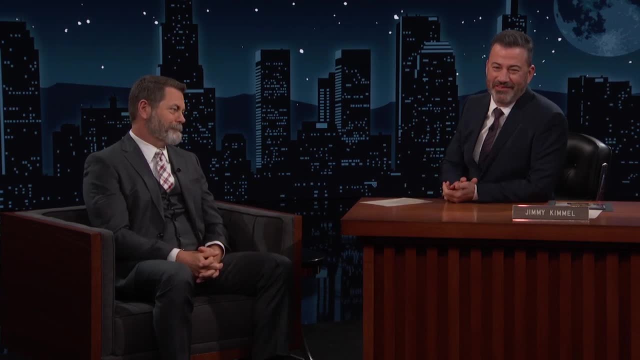 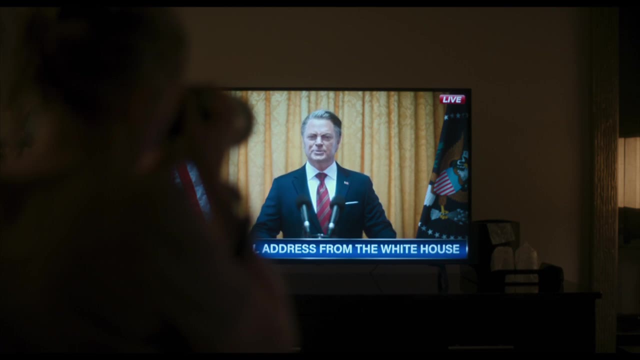 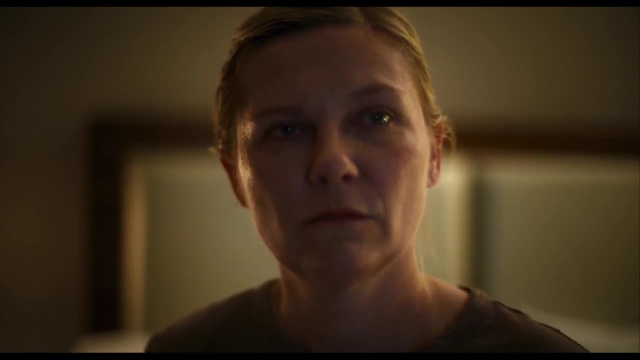 Millsap and weed. Nick Offerman is with us. Civil War is a movie. We'll be right back, Citizens of America. we are now closer than ever to a historic victory As we eliminate the final pockets of resistance. God bless you all. 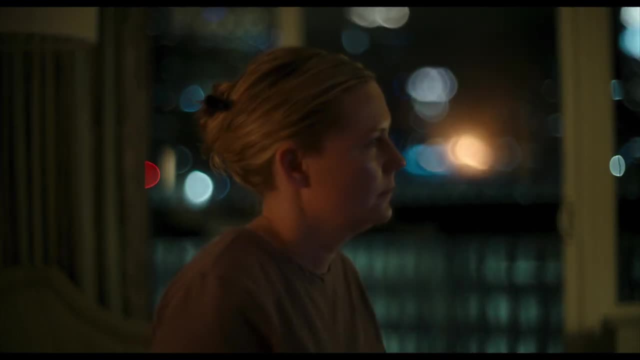 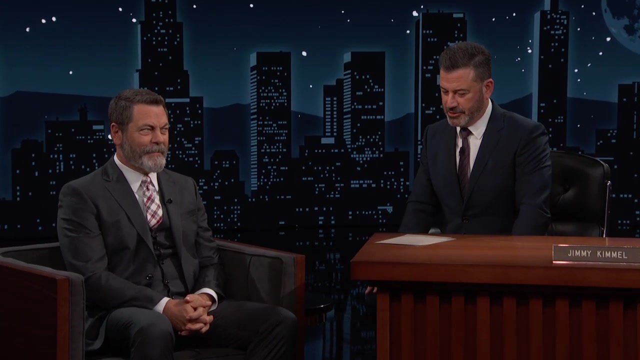 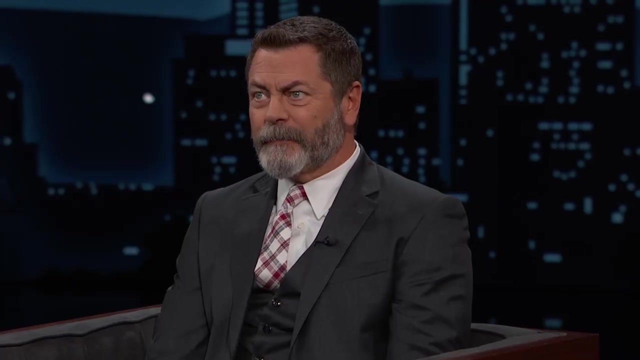 And God bless America. That is Civil War. It is in theaters now. This is Nick Offerman. He's in our studio right now. You got the number one movie in the country. Is that something that registers with you? I mean, that's kind of my thing. 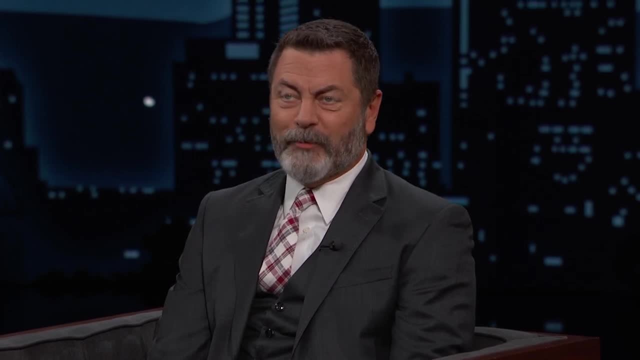 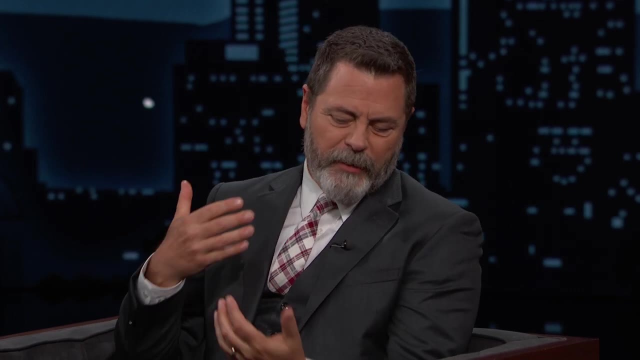 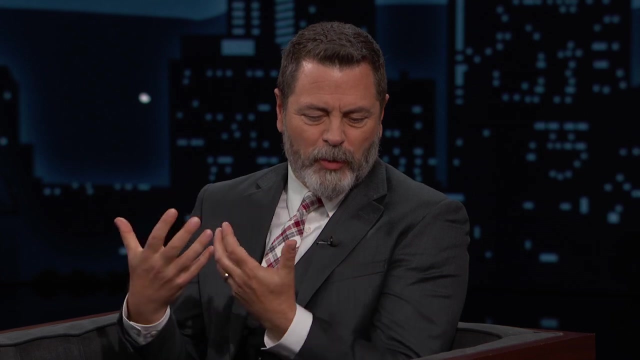 Yeah, No, I am over the moon, especially because I love this filmmaker so much, Alex Garland. He's really underappreciated. He made Ex Machina Annihilation. We did a TV show together called Devs, And now I just think he's an exquisite filmmaker. 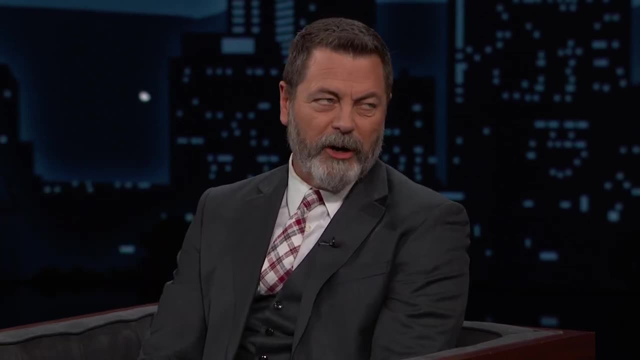 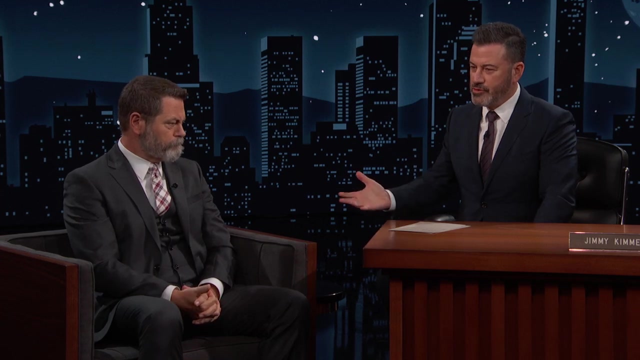 And so I'm so glad that everybody's going to see this. I think it's imperative. Do you feel? besides, obviously it's a compliment To be asked to be in a film that somebody is making? Do you feel an extra good about yourself when they ask you to play the president of the United States? 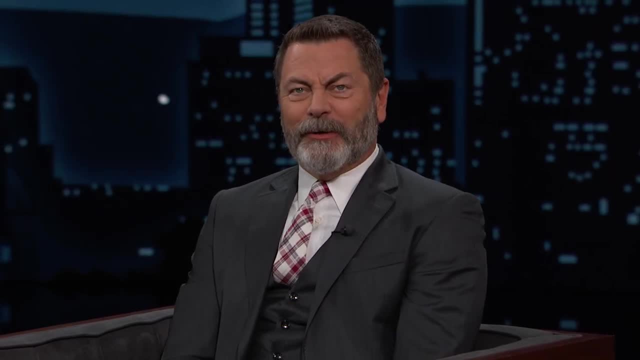 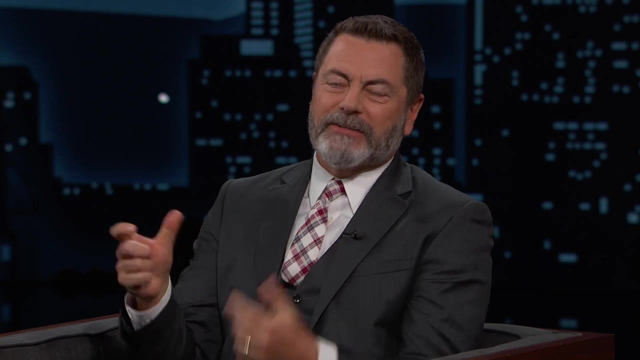 Well, I mean it depends, It really depends. But sure, I don't look at it that way like because it's not that big of a role. I feel I'm kind of like Sauron in the Lord of the Rings. 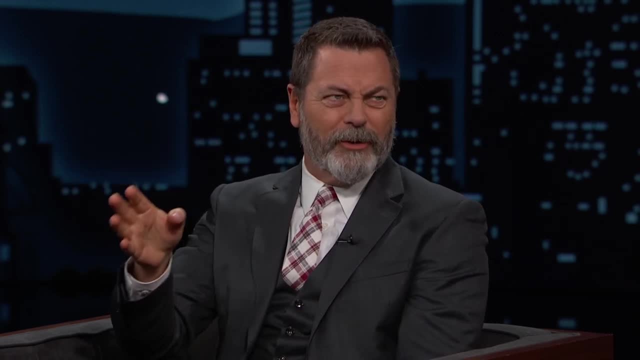 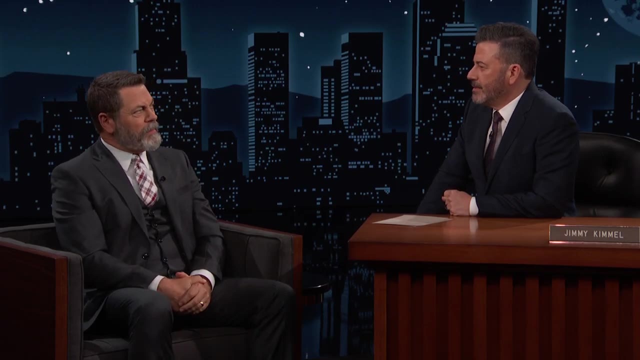 You hear about him a lot and they're always on the way to see him, But you don't really. he doesn't get a lot of screen time. Yes, Yes, And he's not a good president. I mean, he's not a good guy. 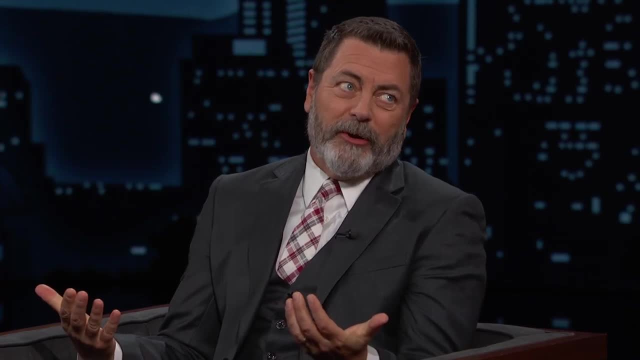 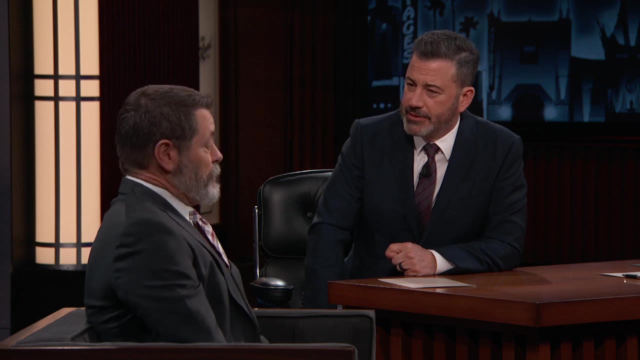 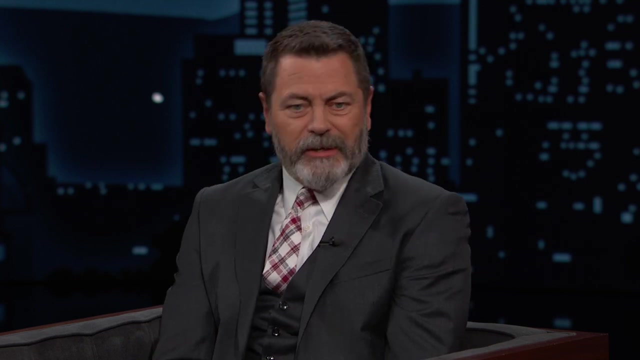 He's not necessarily a good guy. I mean, he's just trying to pay his mortgage, like anybody. Is he based on any of our recent former presidents? No, I mean, there are some details about him that you know he does lean towards fascism. 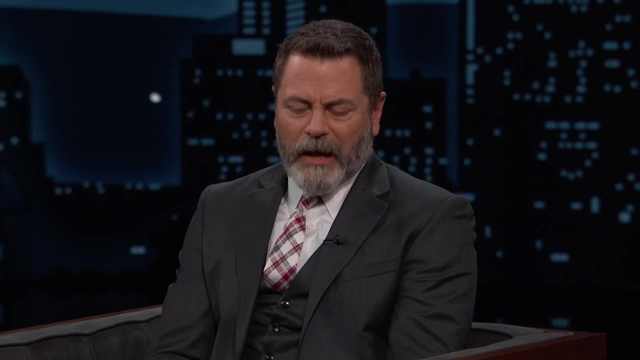 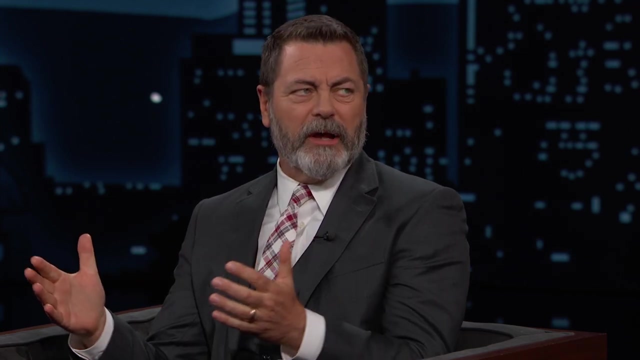 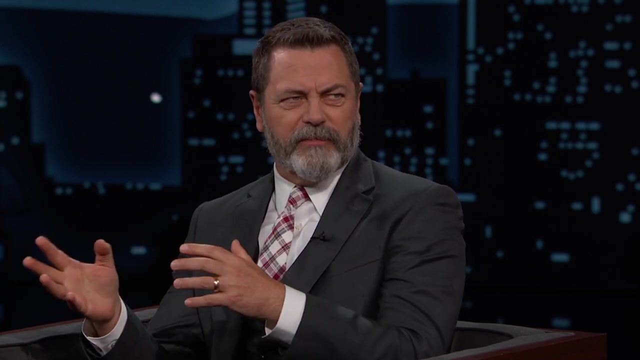 But no, Alex. Alex is very- And it's an important part of the movie actually, that there are. there are no political echoes of real life. It's a, it's a very fictional America And you actually don't know who are in the sides of the war. 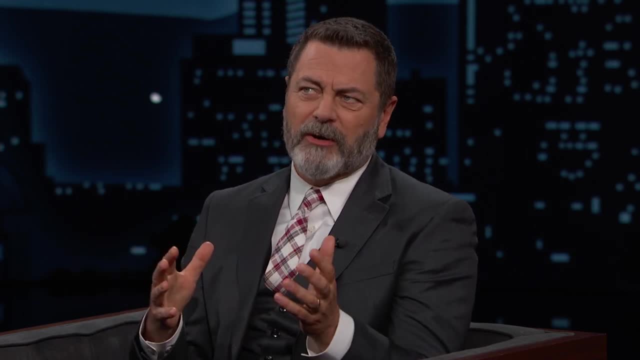 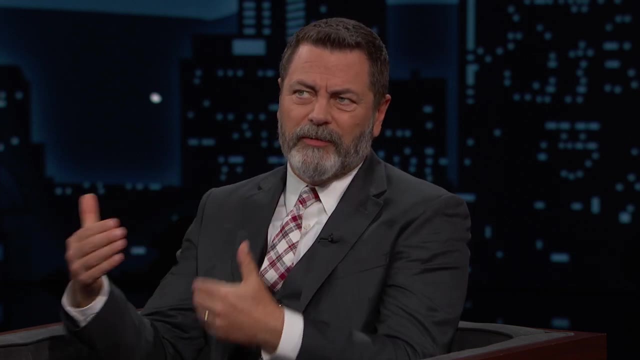 And you don't know my president, You don't know what his politics are, other than he's full of Right, Yeah, Which I mean that could be anybody, And so that's important to the film, because you come out of it having a conversation about: should we? 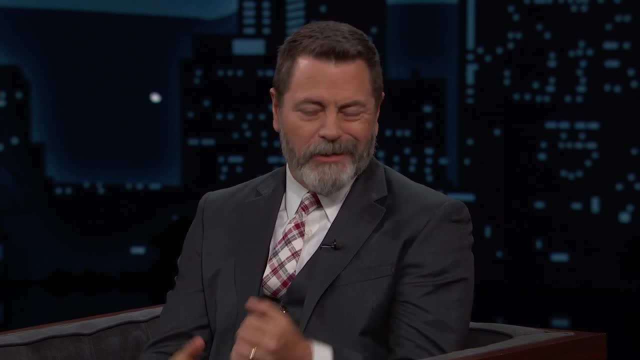 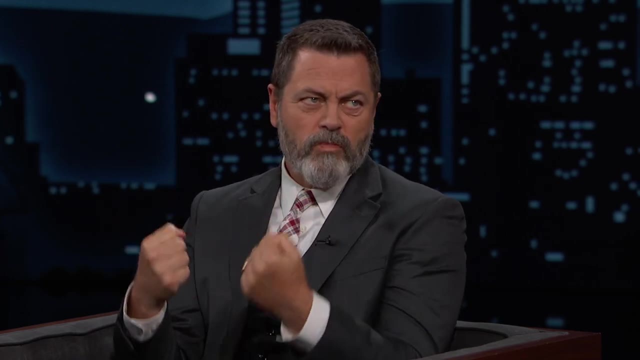 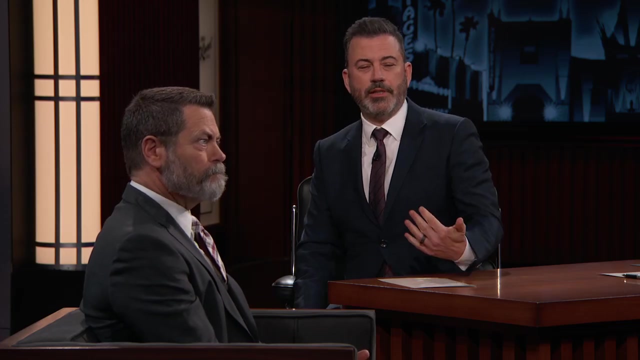 Should we? Should we head towards war versus the devices, conversations of like red versus blue, decency versus red, or you know Mm, hmm, Yeah, And you know, I have to say I feel like, And I hope you take this as a compliment- 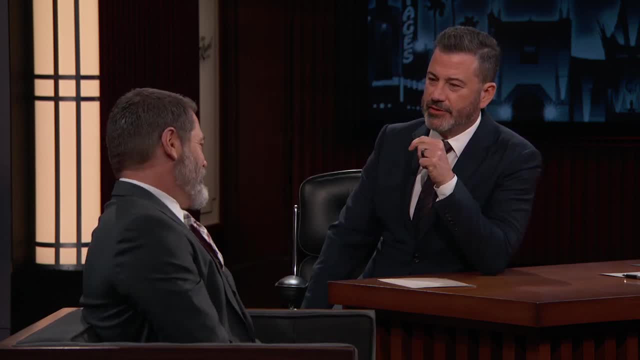 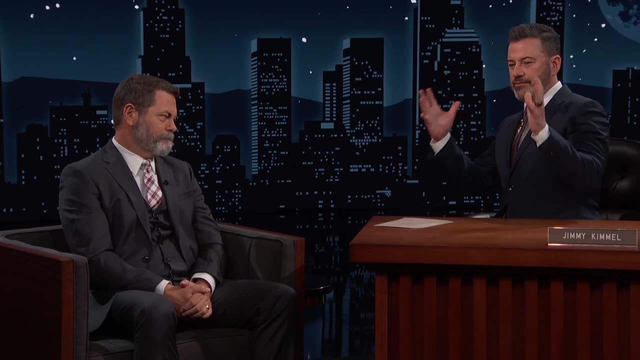 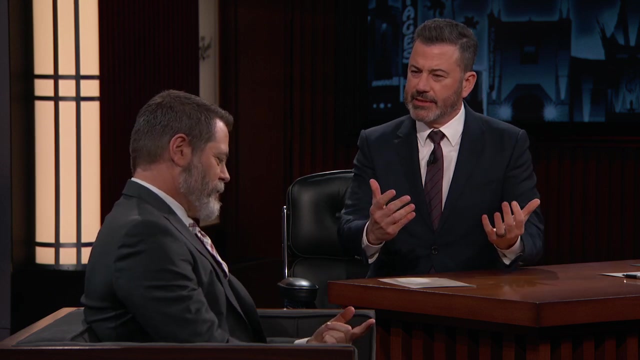 I feel like you could be the actual president if you decided I don't. I don't take that as a compliment, Because I think that you have like you have the Just kind of like the real life credentials, like with your woodworking and whatnot, and working you're like a regular man on time. 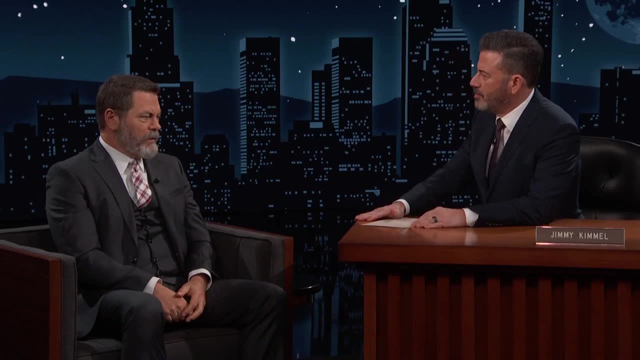 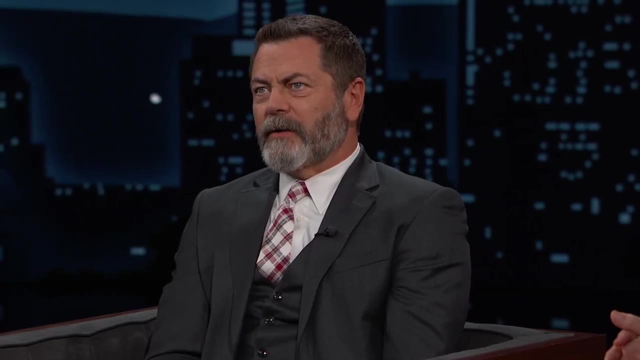 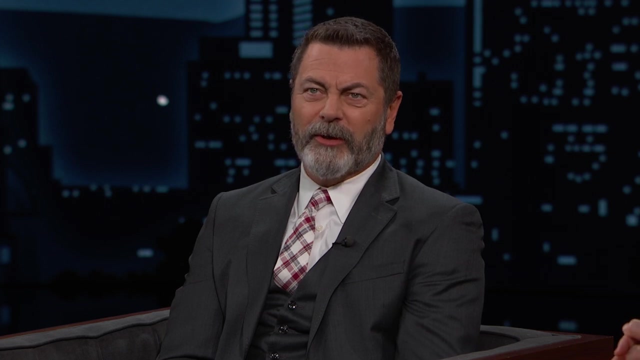 Intelligent and punctual. I mean, what would a Nick Offerman presidency be like? Have you thought about that? I Well, I mean, I have thought about that. Sure, I would pay a lot of attention to our agriculture. I'm going to answer you earnestly. 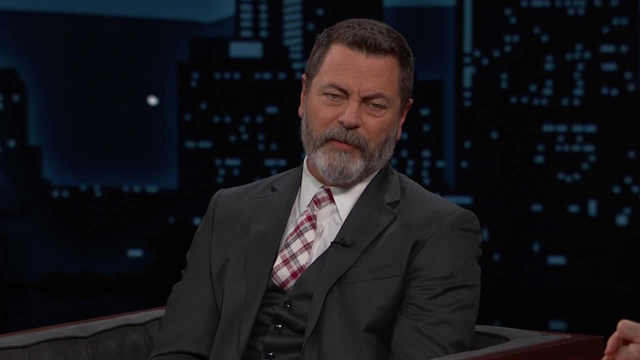 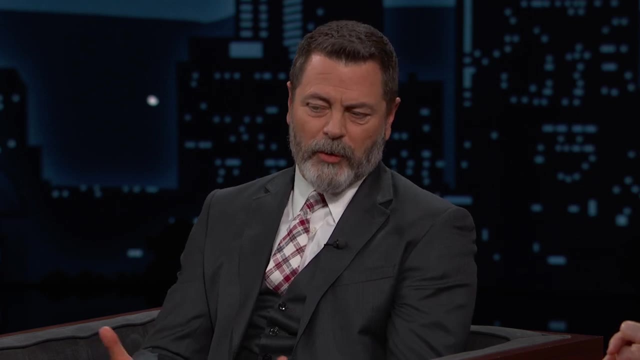 OK, I would urge. I would urge our government to pass a new farm bill that pays attention to our farmers, who are providing all the food that we eat and who we've come to ignore in this industrial time. All right, All right Good. 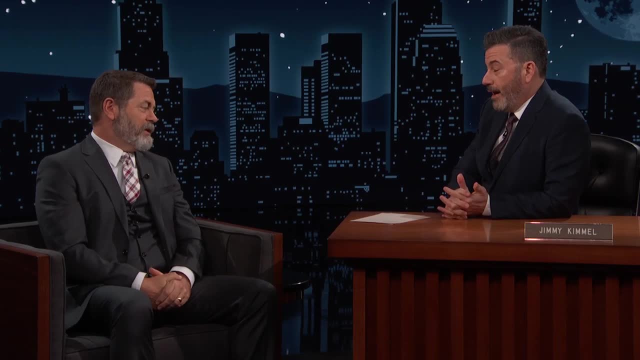 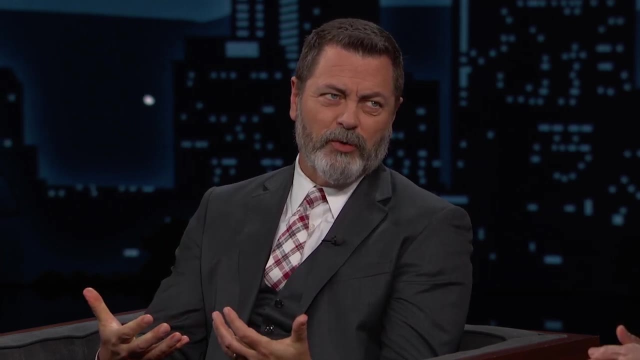 Yeah, I mean, it's not super sexy TV to talk about soil health, but I would also reinstate woodworking and kitchens and sewing in our schools and teach our kids So how to make things with their hands. Now do you? do not have woodchop. 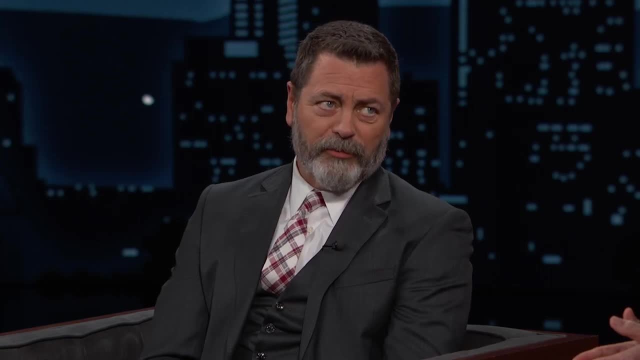 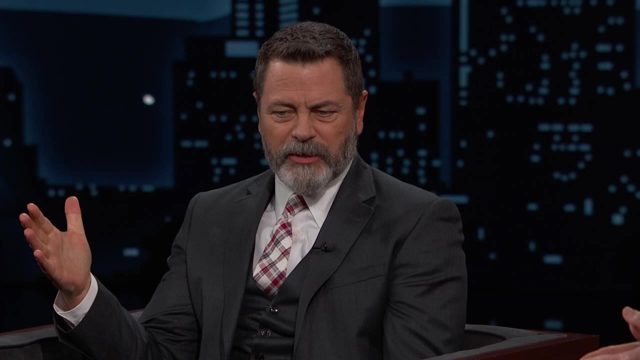 Do you have a metal shop in school anymore? Not, not to. most schools have done away with all of their shops and their home economics. like learning to, to cook, I mean all of those things I love to cross the board. I loved learning to make casserole and I loved learning to build a table. 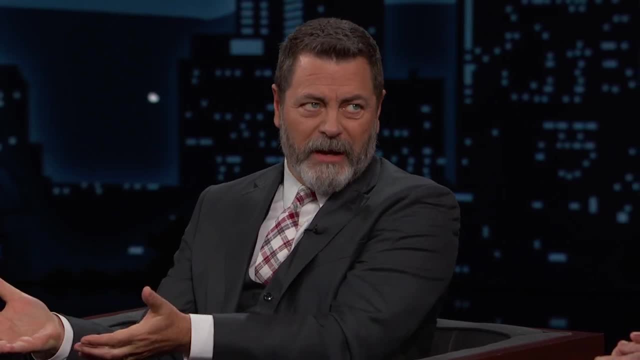 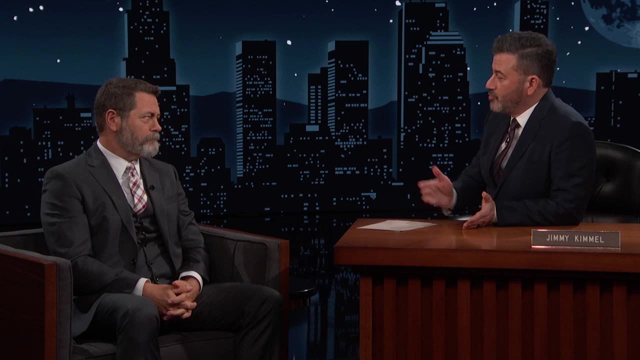 All of those things you need. if you want to serve casserole, you need a table. 100 percent, You can't eat a casserole on the floor. No, So you took. you were one of those guys in our school. 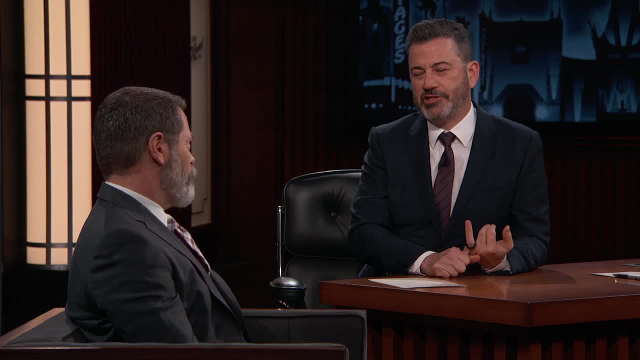 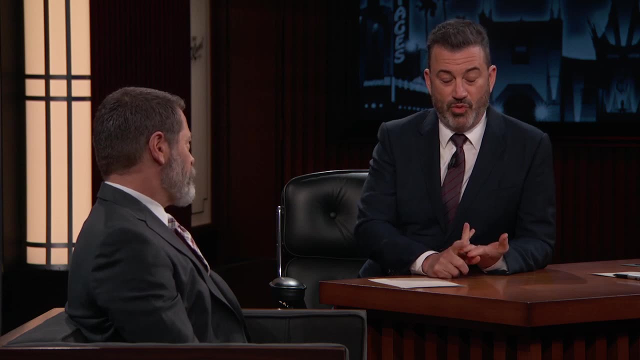 Like they can't. Kids who took- OK, kids who took- wood shop or metal shop really just wanted to make a bong in class, Sure. And then the kids who took home act just wanted to have a snack because they just made a bong in class. 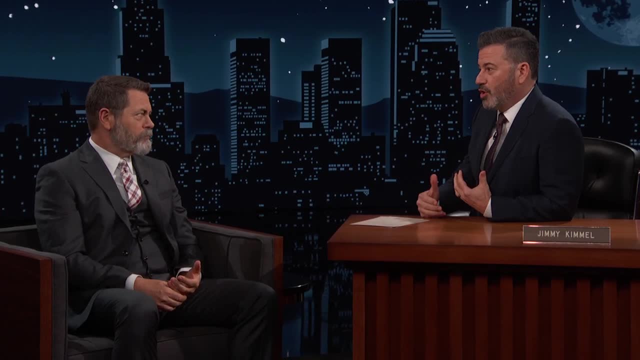 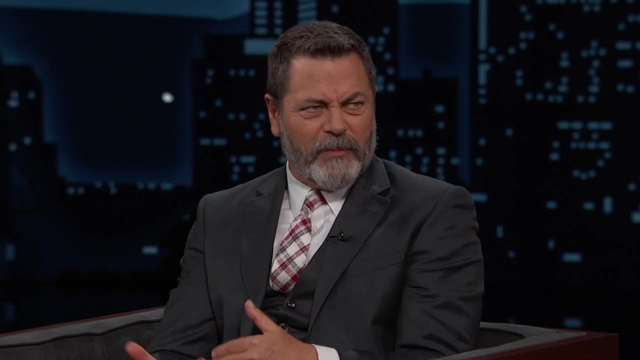 That's right, And that was kind of none of them necessarily were looking to do it. What you've just described is a healthy economy. It's moving, We need resources And you end up with a happy constituency. You do Yeah.